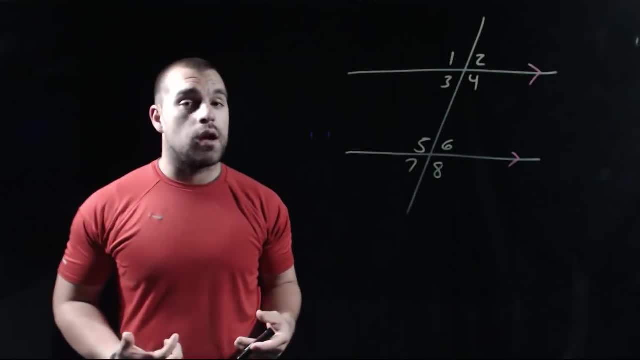 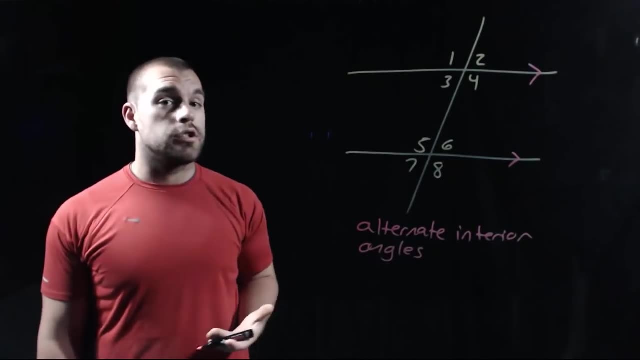 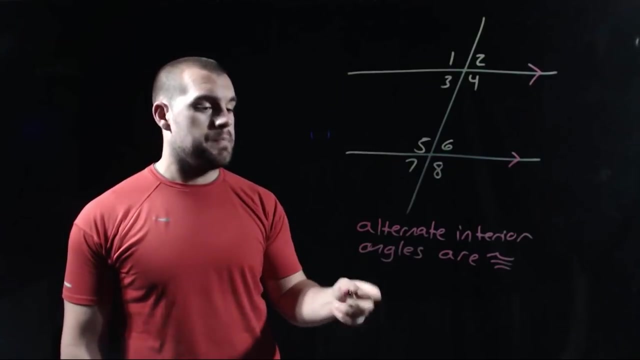 angles. Our next pair of angles that we talked about in 3.1 is the angle of the transverse. So we talked about were alternate interior angles And their relationship is that these are also congruent. So we've got two pairs of alternate interior angles in our picture. 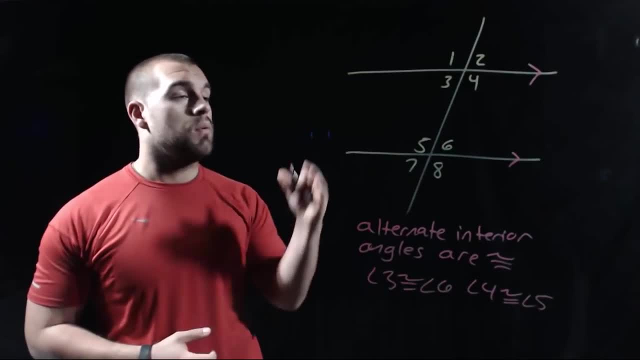 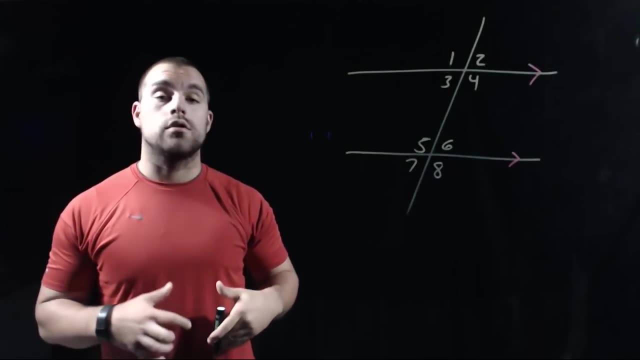 We've got angles 3 and 6.. Those things are going to be congruent. And we've also got angles 4 and 5.. Those angles are also congruent. Our next angle pair that we talked about was alternate exterior angles. 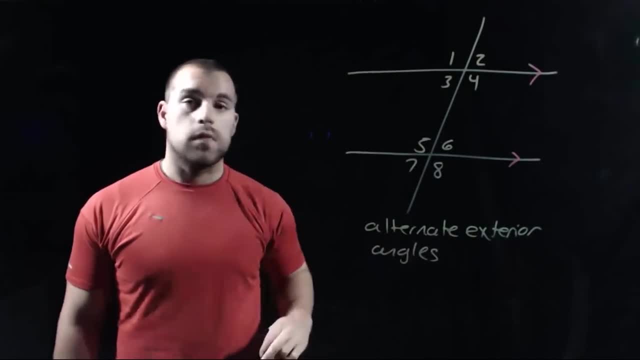 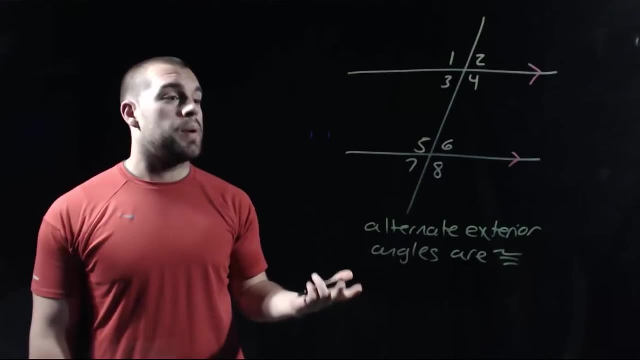 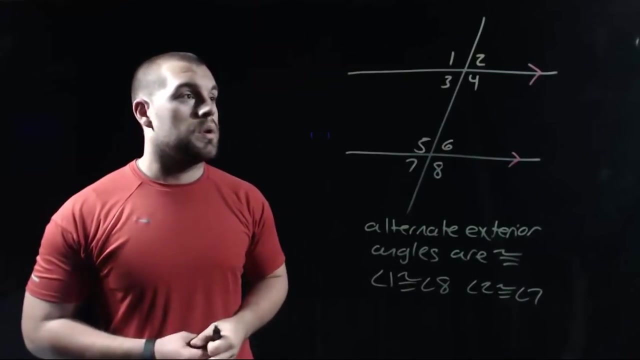 And much like the other angle pairs that we've talked about so far, these are also congruent. So in our picture we've got two pairs of alternate exterior angles. We've got angle 1 and angle 8. Those are congruent. And we've also got angle 2 and angle 7. Those angles are congruent. 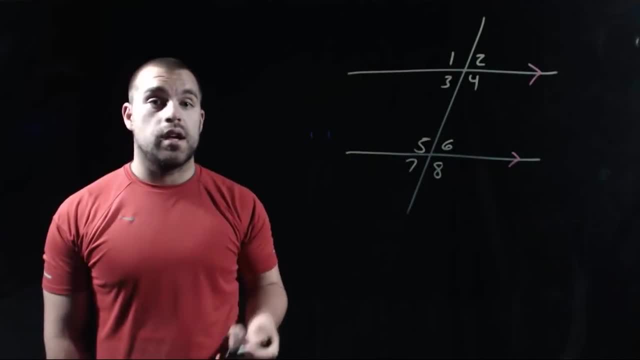 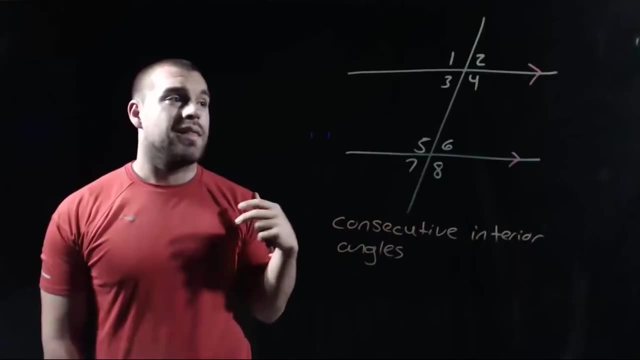 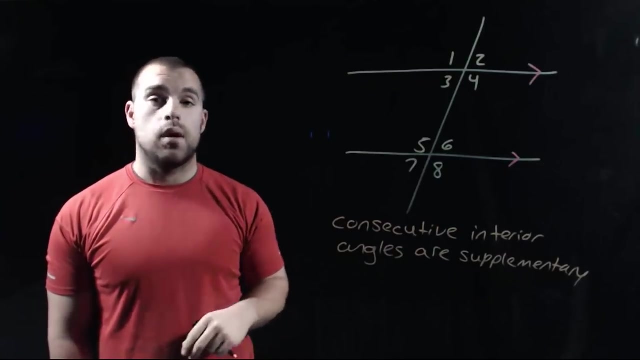 Our last angle pair was consecutive interior angles. These ones are going to be congruent. These ones are different. These are supplementary And remember, supplementary means they add up to 180 degrees. So we've got two pairs of consecutive interior angles. We've got 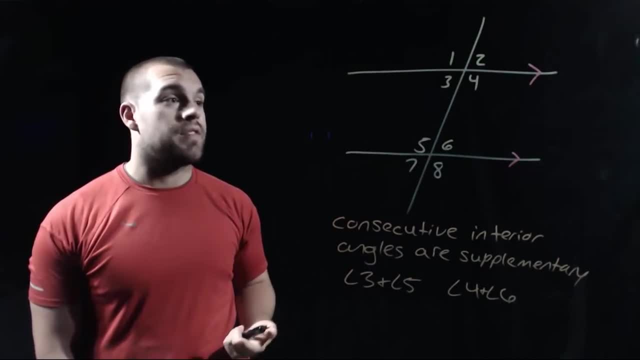 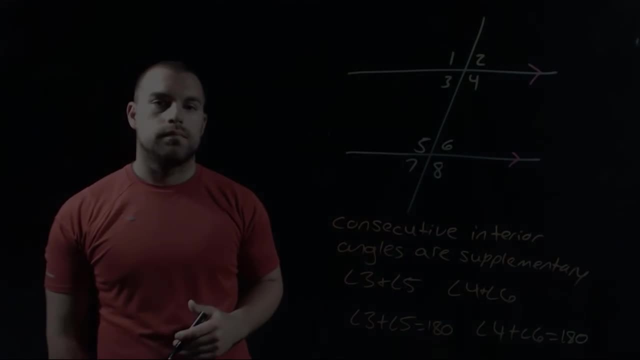 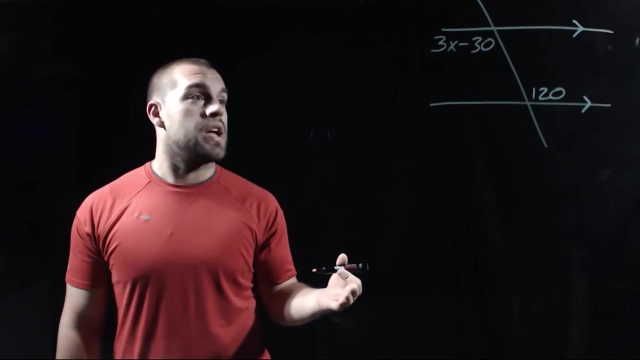 angle 3 and angle 5, and we've got angle 4 and angle 6.. Those pairs of angles will add up to 180 degrees. So let's take a look at this example. We've got two pairs of successive parallel lines and we're looking at the measure of two of those angles. 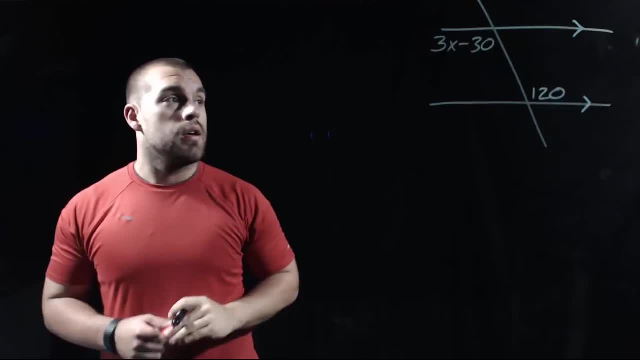 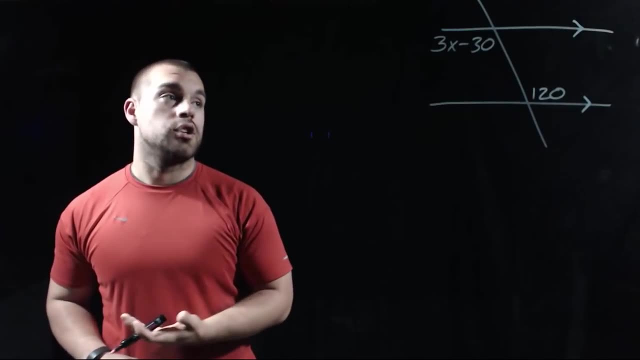 Over here we've got 3x minus 30, and down here we've got 120.. First thing we're going to decide is: what kind of angle pair is this? Then, based on that angle pair, we'll look at the relationship between the angles and set. 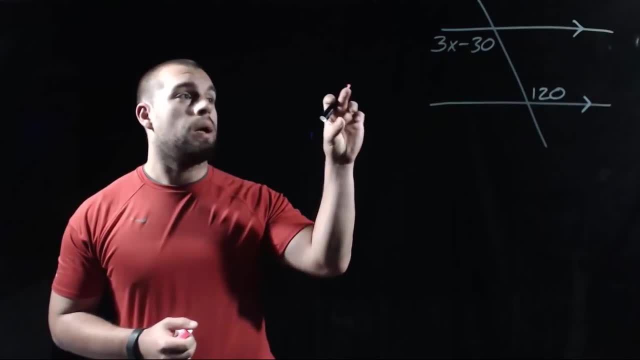 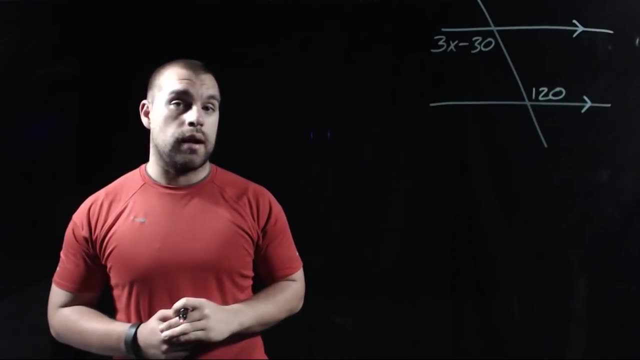 up an equation that we can go through and solve. So, if we take a look at these, these are two angles that are between those two parallel lines and on opposite sides of the transversal. So these are alternate interior angles. And remember the relationship between alternate interior angles when our two original lines 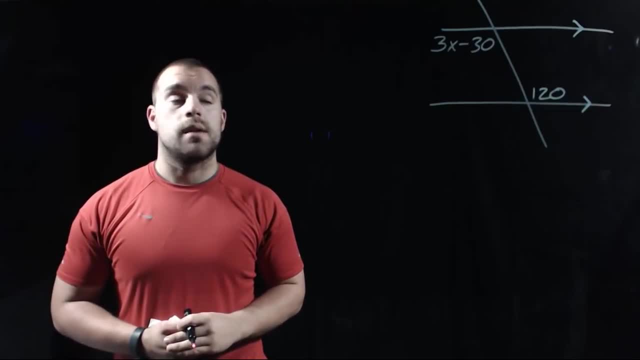 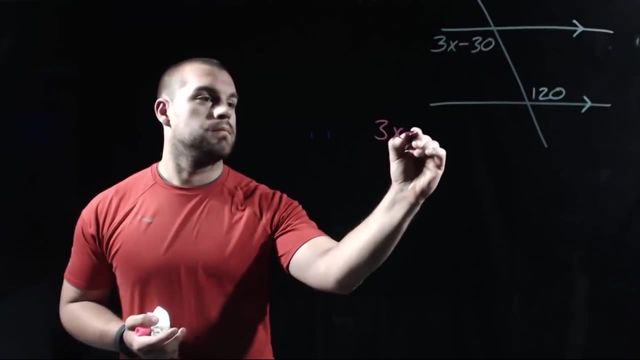 are parallel, those two angles are congruent. So if we're going to set up an equation that we can go through and solve, the angles being congruent means that their measures are equal. So we can set up an equation that says 3x minus 30 equals 120, and then we're just going.